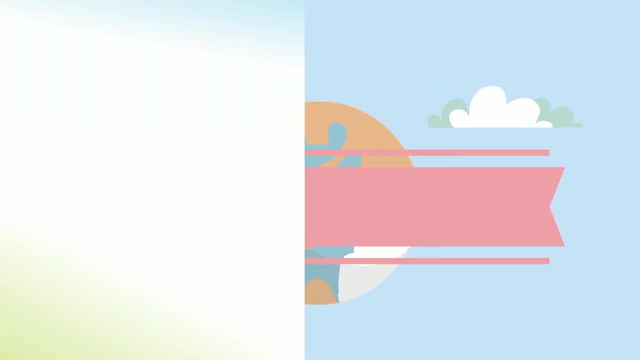 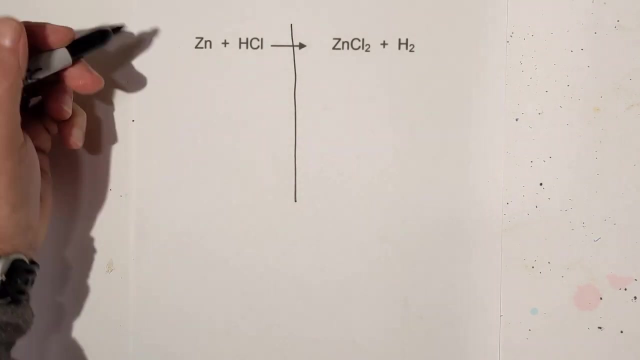 Welcome to MooMooMath and Science. In this video, let's balance some equations. So let's get started. Step one I like to do is just draw a line down the middle and then count atoms. So let's go ahead and start. We have zinc and it looks like we have one. 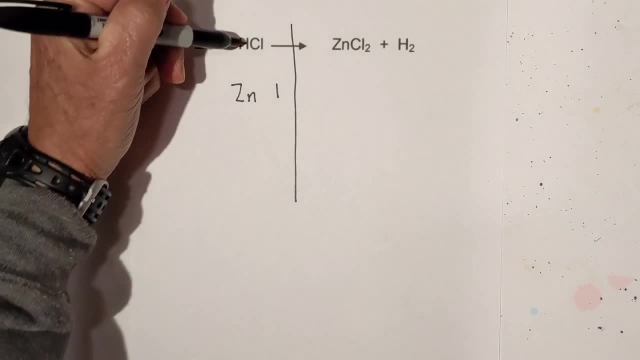 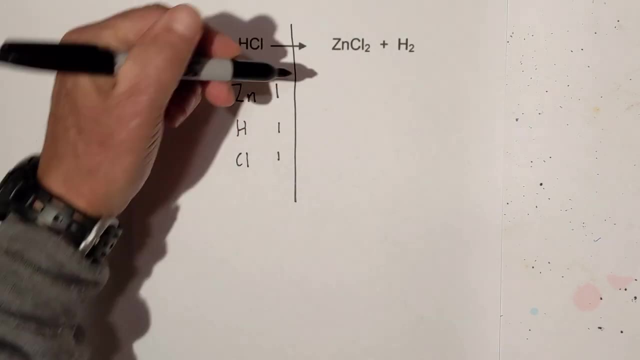 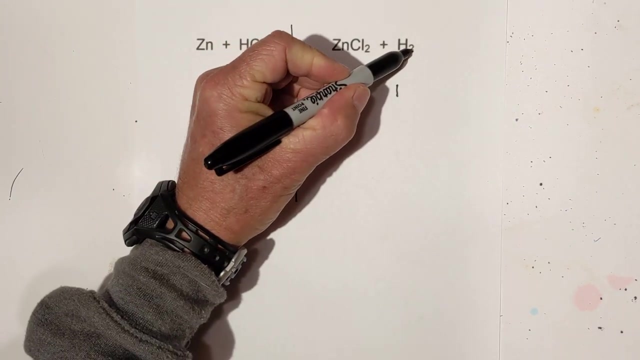 Remember, anytime you have a capital letter, that means you have a new element. We have hydrogen and we have one of those. and then we have one chlorine, One of those. Okay, let's do the same on this side. We have zinc- looks like we have one Hydrogen. remember a subscript. 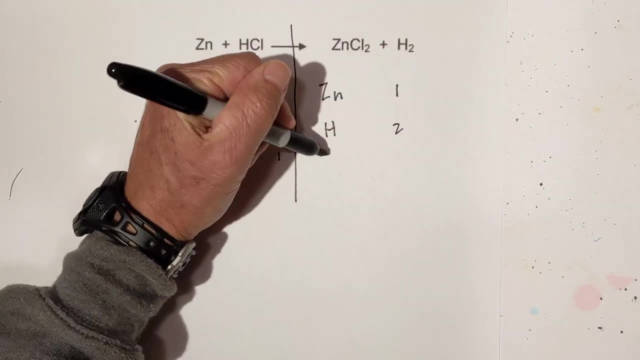 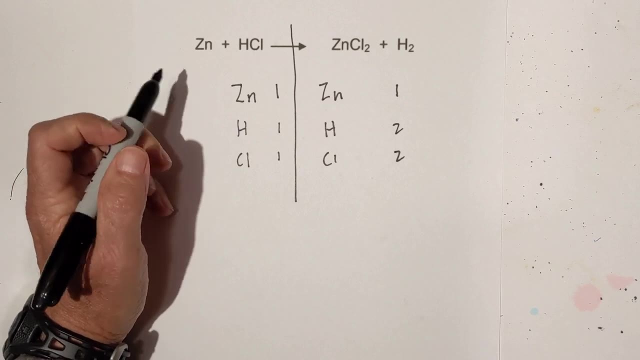 applies only to that element. We have two of those and then it looks like we have two chlorines. So now I begin with the metals and then I go non-metals and then I go other, including hydrogen, So it looks like the metals are balanced for right now. 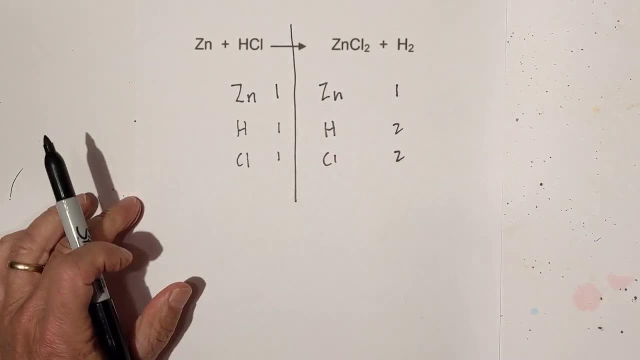 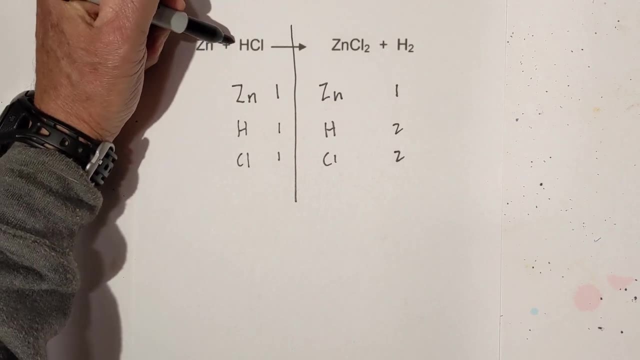 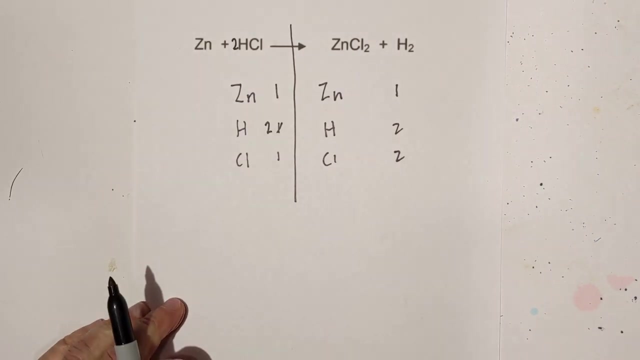 Hydrogen. we have one on this side, two on the other, So the only thing I can do is I can add a coefficient to the beginning. Okay, so I am going to apply a coefficient here. So that means we now have two hydrogens and we have two hydrogens, So they are balanced. 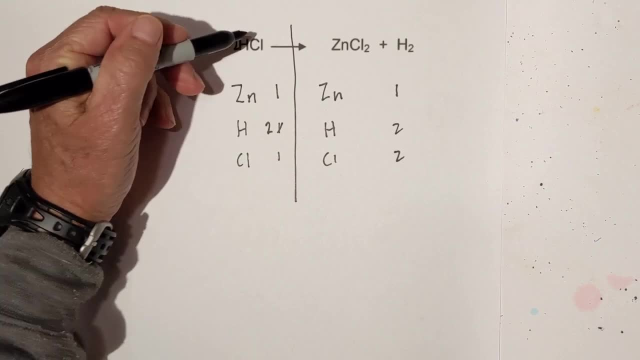 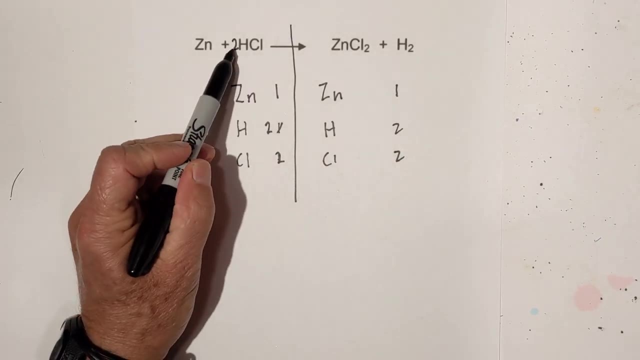 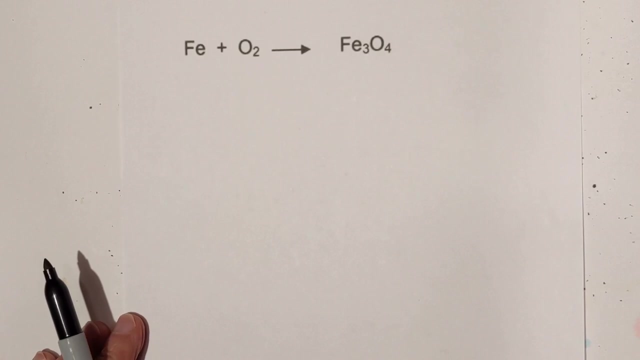 But now the chlorine. when we multiply two times one, we have two chlorines, and guess what? it's in balance. so there it is. all we had to do was add a two right there. okay, let's work on another one, okay. so now let's try this one. draw a line down, let's count atoms. um, we have. 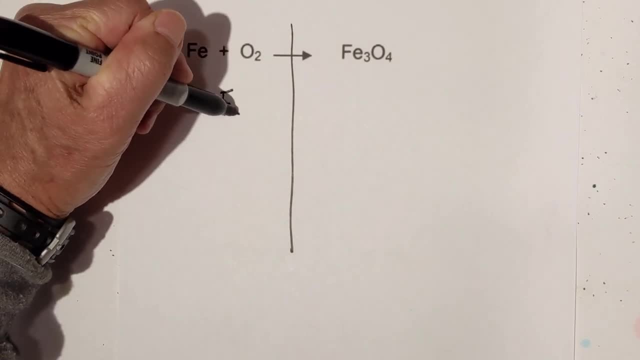 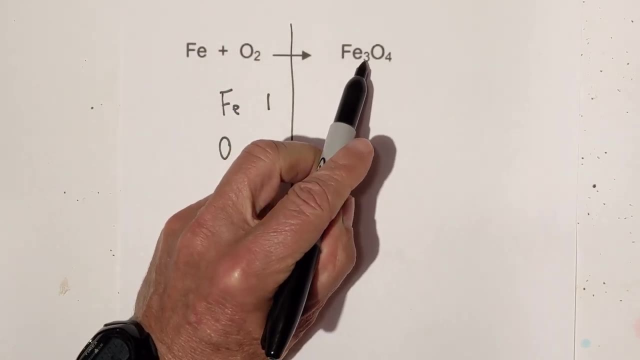 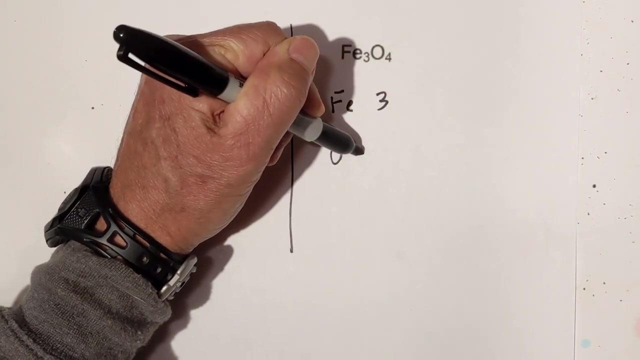 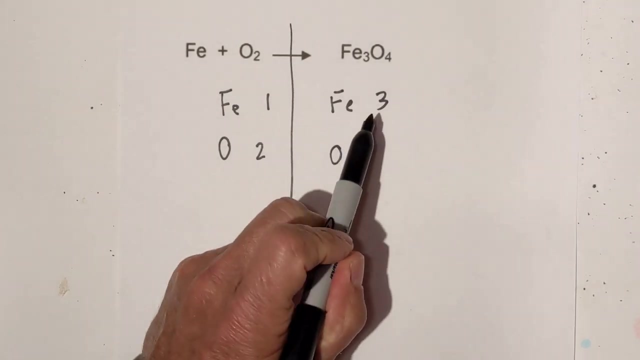 um iron here, and so it looks like we have one iron and two oxygen and on the other side- uh, remember, the three only applies to the iron. so we have um three on this side and then we have four oxygens. okay, so let's start with the metal. always start with the metal first, and we have 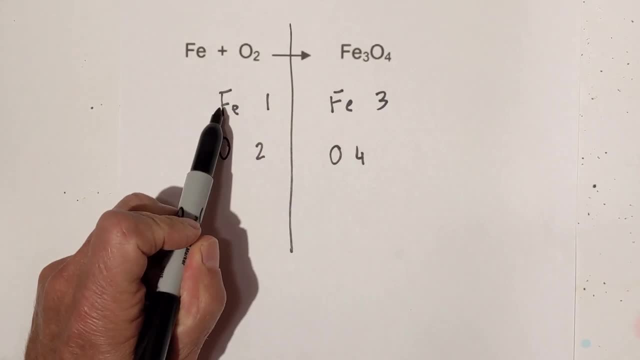 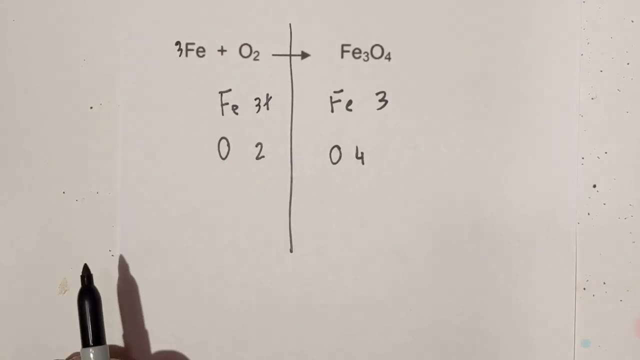 three on three on this side, one on this side, so i can add a three to multiply it by there. so three times one is three. so now the metals are balanced. but now let's look at oxygen. and we have two on this side, four on the other. so what i do? 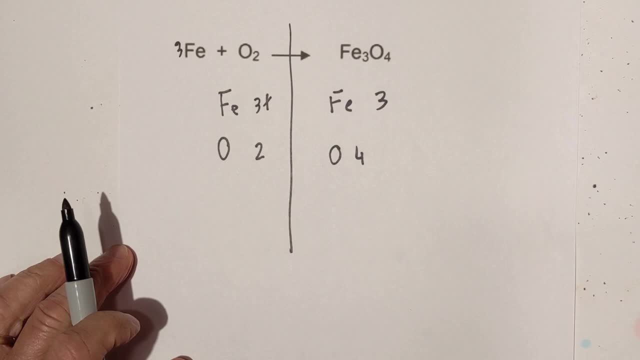 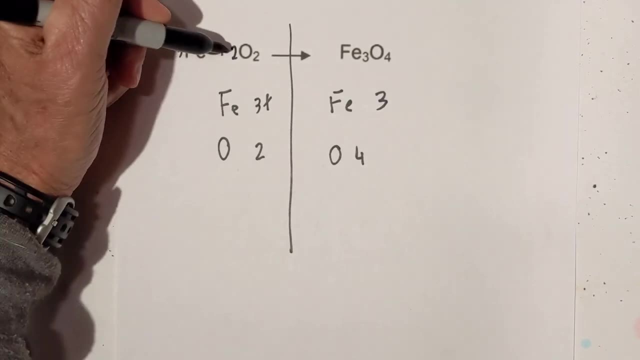 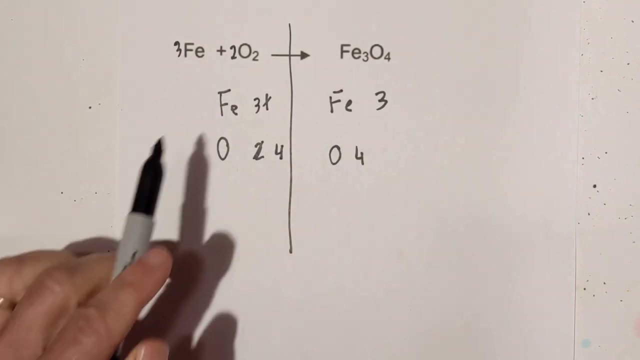 next is: what's the smallest number? these, both of these numbers will go into and that is a four. so if i multiply two times two, that is four. so now that is four and it looks like we have three and four. so again, pretty simple, um, and it's balanced. let's try one final one. 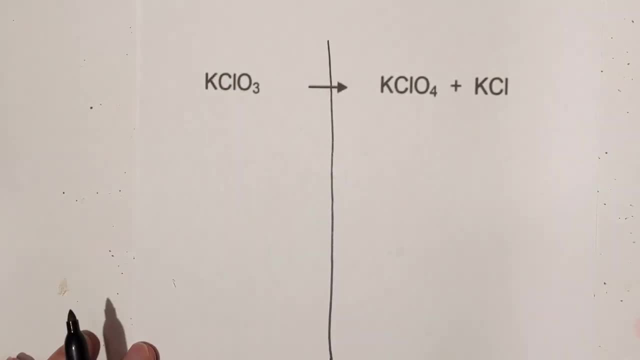 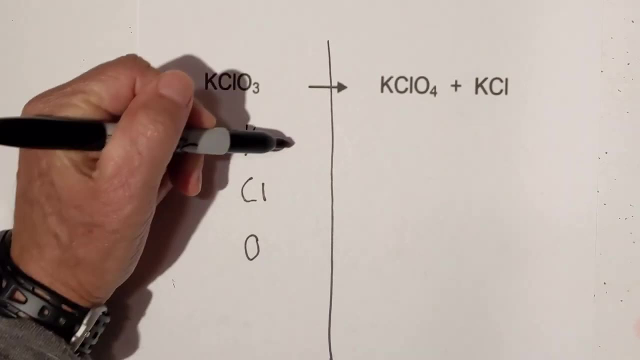 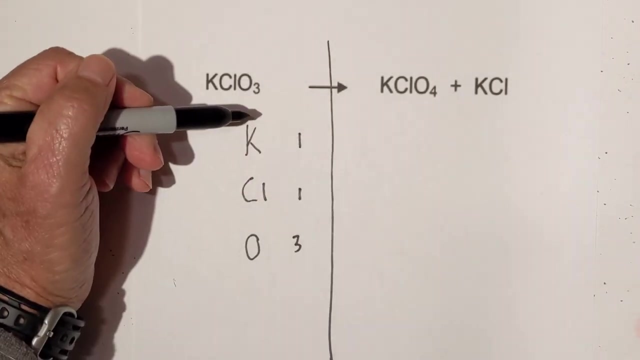 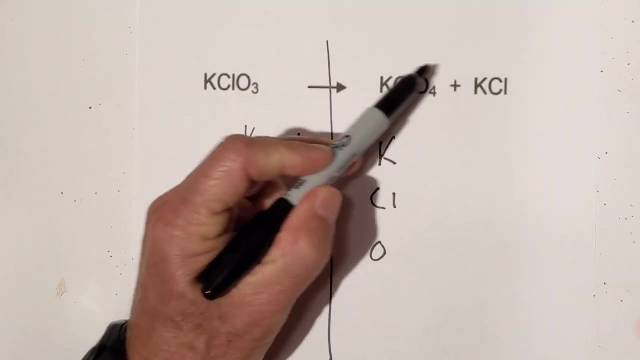 okay, last one, draw a line down. let's separate the elements out. okay, let's count. we have one potassium. we have one chlorine. we have three oxygens. now on this side, let's do the same. we have um potassium, chlorine and oxygen. we have two potassium, so i'm gonna write it two there. it looks like we have chlorines. 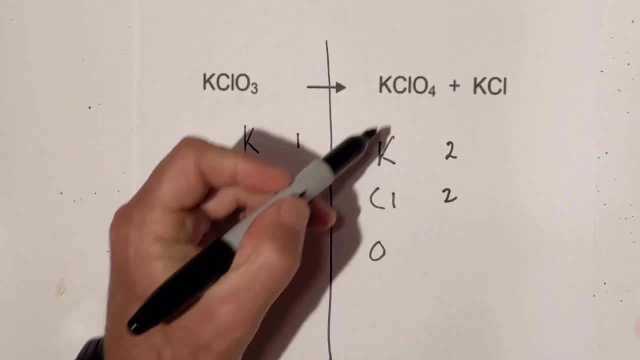 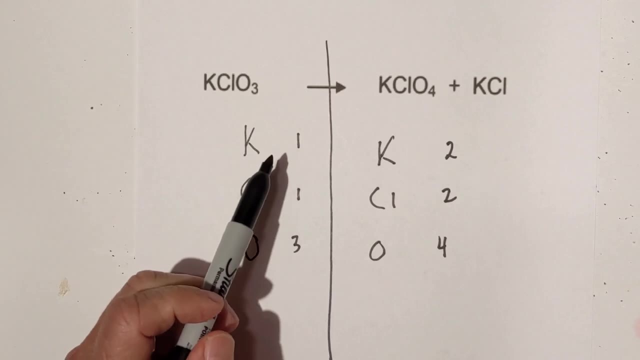 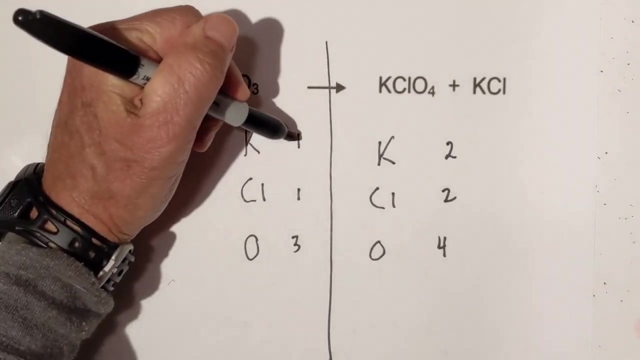 we have one here and one there, so we have two of those, and then we have four oxygens. so now let's see what's balanced. well, let's start with the metals. and um, we have one and two, so i'm gonna multiply this by two, so this becomes two. but now the chlorine becomes two. 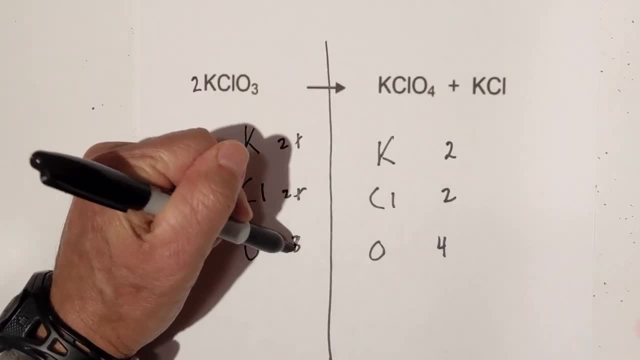 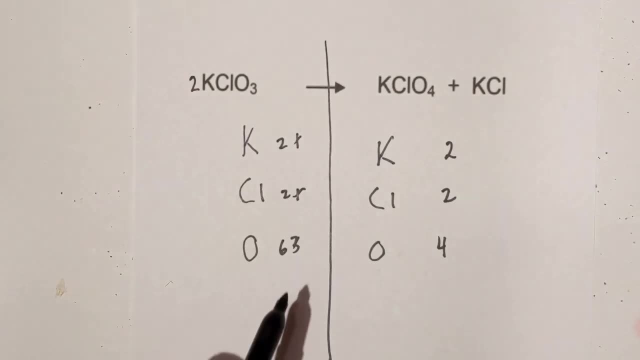 and then two times three. okay, two times three, that becomes six. so so the potassium's chlorine. they're all balanced, but now i have a problem with the oxygen. we have six and four, so again i go back to what's the smallest number. both of these numbers will go. 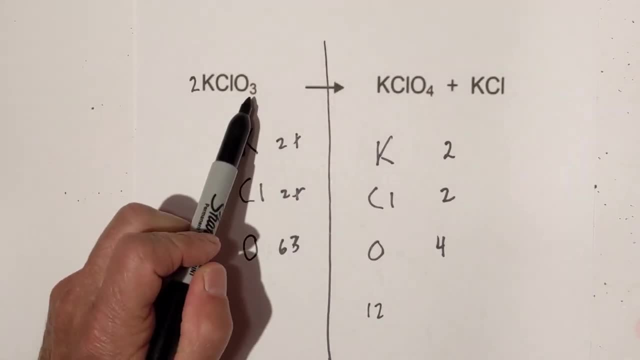 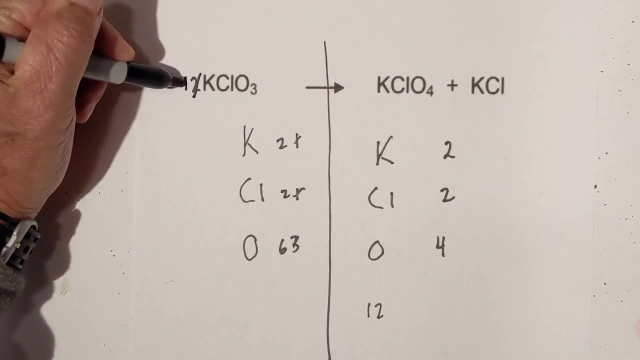 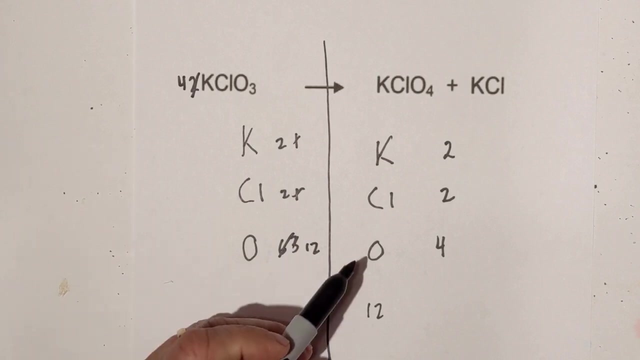 into and that is 12.. i have a subscript of three. three goes into 12, how many times? and that is four. so i'm now going to have to change this to a four. so four times three is we have this as 12.. okay, so. 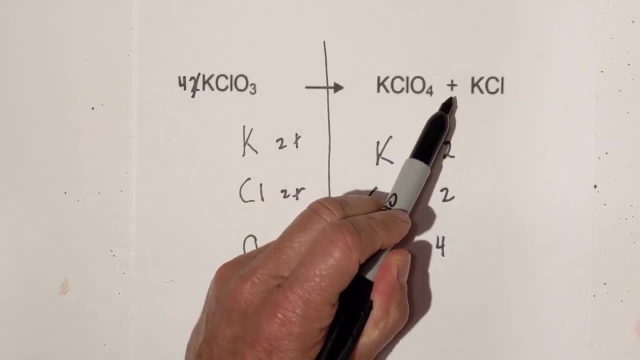 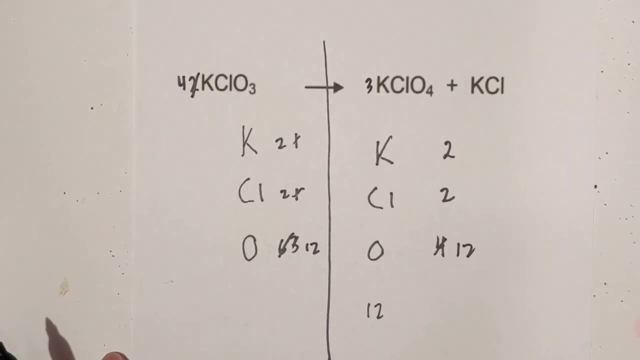 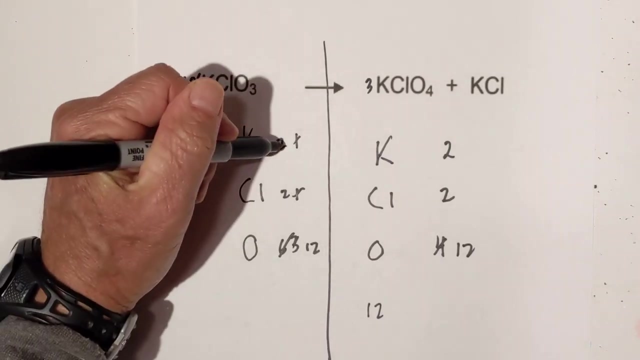 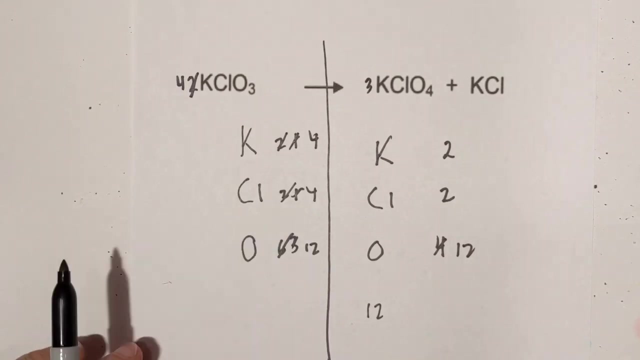 let's go to the other side. four goes into 12 three times so. but now we've got to reset because we have a different number in front. so now we take four times one, because assume that there's a one there. so now we have four potassiums, we have four chlorines and then we have 12 oxygens. now let's 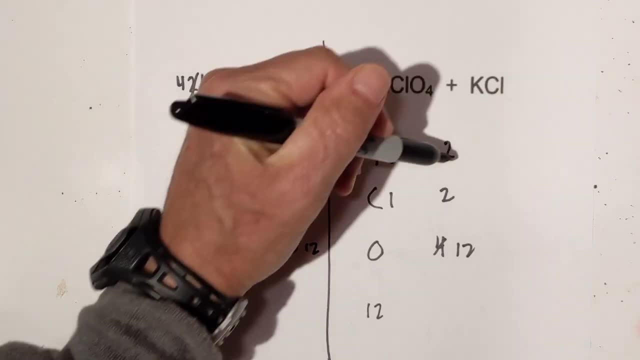 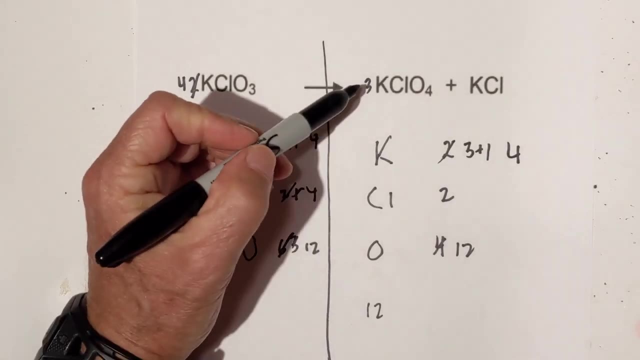 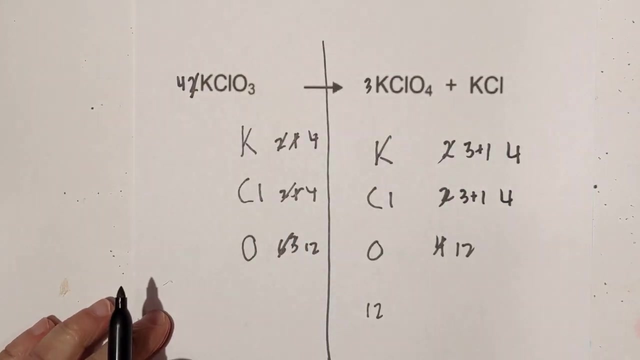 see what we have on the other side. we have, uh, potassium plus one, so we have four. we got pretty lucky there. and then we have three chlorines plus one, so it'd be three plus one, so we have four there. and then we have three times four, which is twelve. so it is now balanced, okay, and we had to add a four here. 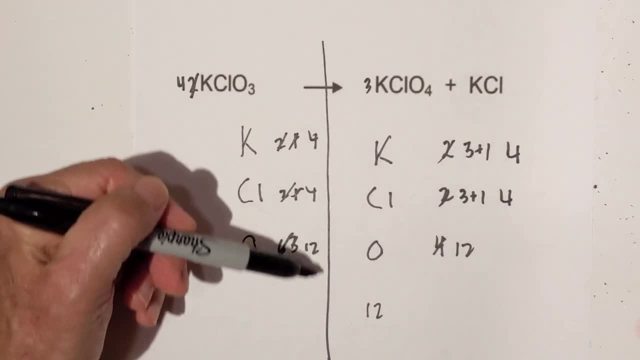 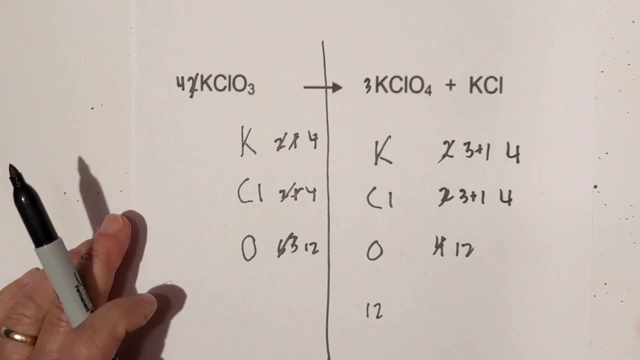 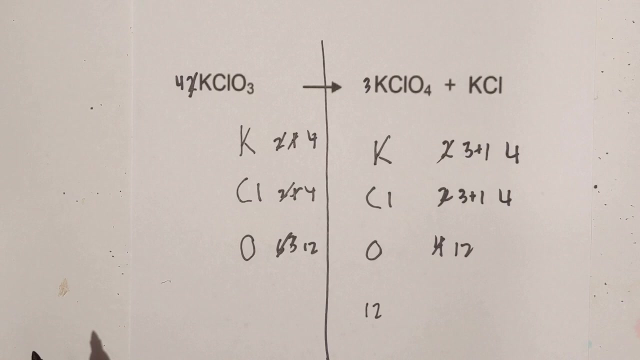 and a three on this side. so, in summary, i draw a line down the middle, i count atoms, i then start with my metals, then i go non-metals and then i go hydrogen or if you have anything else. i hope that helps and remember: kindness multiplies kindness. be kind to someone today. 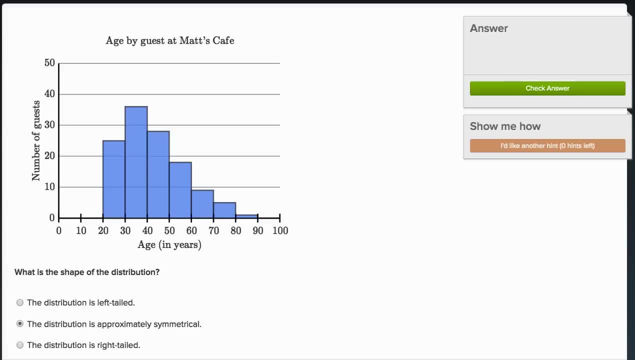 So what I want to talk about now are shapes of distributions and different words we might use to describe those shapes. So right over here, let's see, we're talking about Matt's Cafe and we have different age buckets, So this is a histogram here. 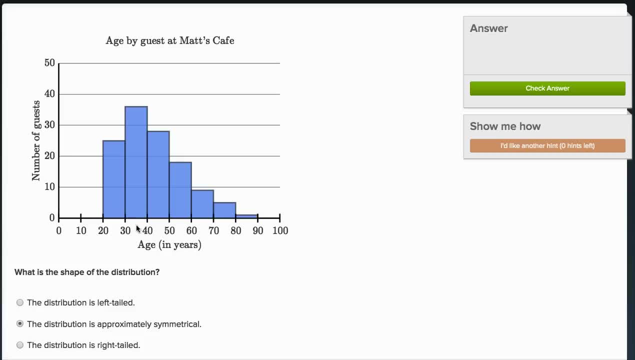 And in each bucket it tells us the number of guests that are in that age bucket. So a lot of. we don't have any guests that are under the age of 20.. We have a reasonable number between 20 and 30. We have a lot of guests at 30,. 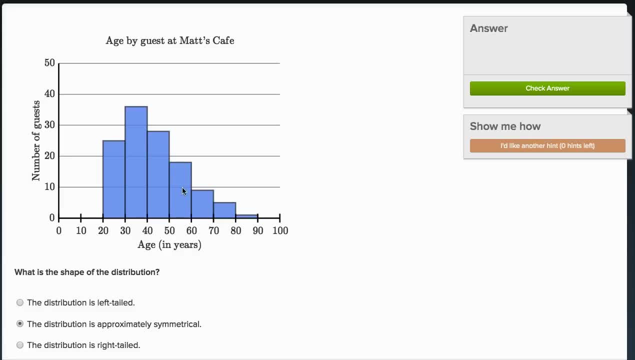 in that bucket between 30 and 40. Reasonable number, between 40 and 50. And then, as we get older, we have fewer and fewer guests. So just when you look at something like this, a distribution like this, something might pop out at you. 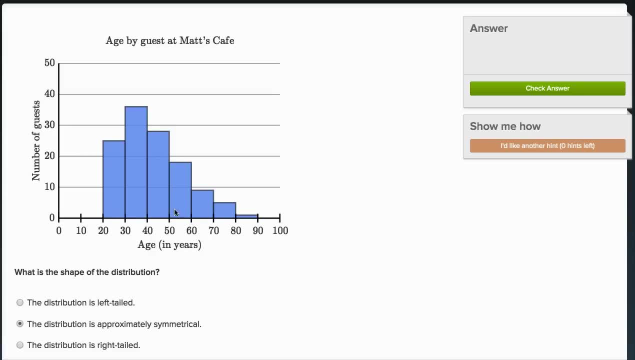 It kind of looks like if you were to imagine this were an armadillo, this would be the body of the armadillo, And then what we see to the right kind of looks like the tail of the armadillo, And we actually use those types of words.